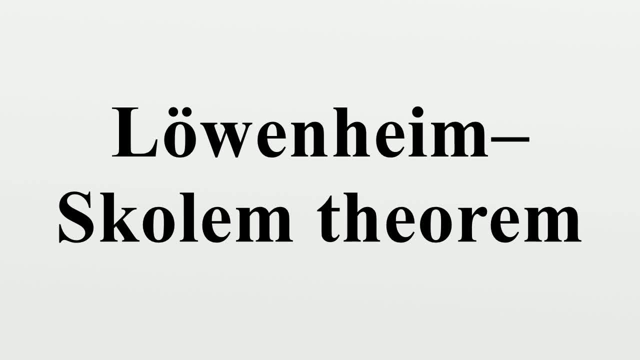 an interpretation of a constant symbol and a function symbol of σ in M is simply an element of M. More generally, an interpretation of an nary function- symbol f- is a function from Mn to M. Similarly, an interpretation of a relation- symbol r is an nary relation on M, ie a subset of Mn. 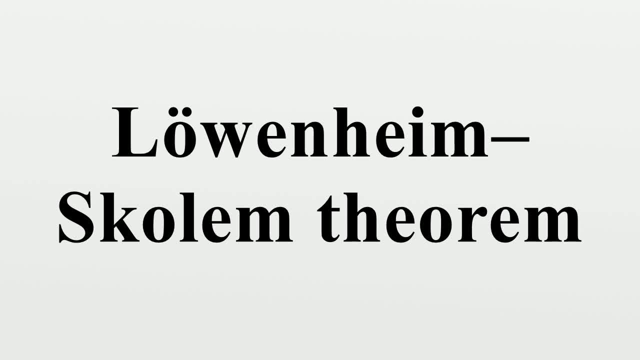 A substructure of a σ structure, M, is obtained by taking a subset N of M, which is closed under the interpretations of all the function symbols in σ, and then restricting the interpretation of the function symbol. In this case, an elementary substructure is a very special case of this. 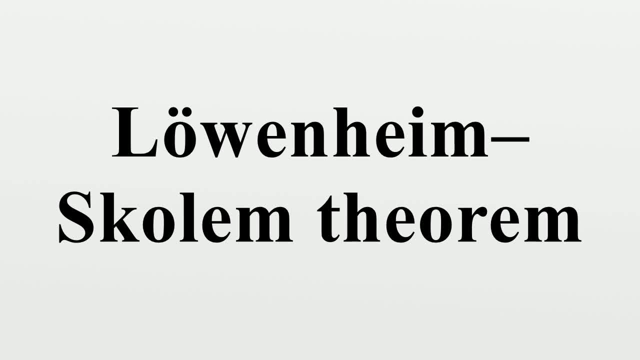 In particular, an elementary substructure satisfies exactly the same first-order sentences as the original structure Precise statement. The modern statement of the theorem is both more general and stronger than the version for countable signatures stated in the introduction. In its general form, the Loewenheim-Scholem theorem states that: 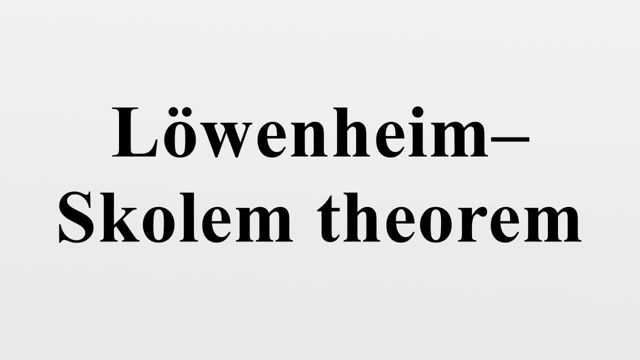 for every sub-structure, there is a sub-structure that is equal to the number of sub-structures. For every signature, σ, every infinite σ-structure, M, and every infinite cardinal number, κ, σ, there is a σ-structure or n such that n equals κ, and if κ less than m, then n is an elementary substructure of M. 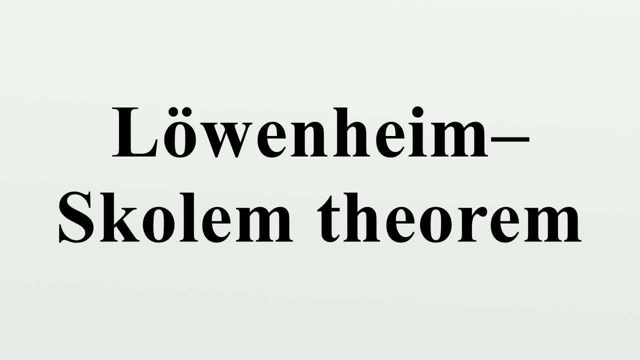 If κ greater than m, then n is an elementary extension of M. The theorem is often divided into two parts corresponding to the two bullets above. The part of the theorem asserting that a structure has m is an elementary substructure of M. The part of the theorem asserting that a structure has m is an elementary substructure of M. 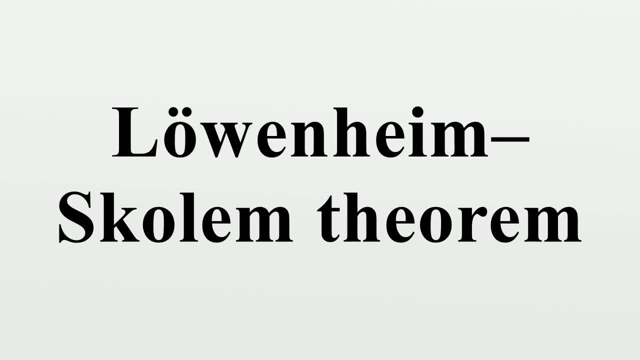 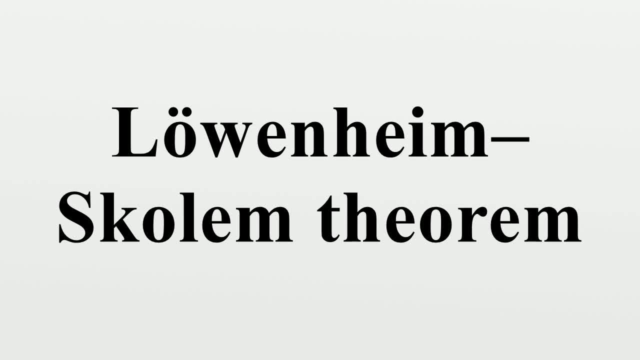 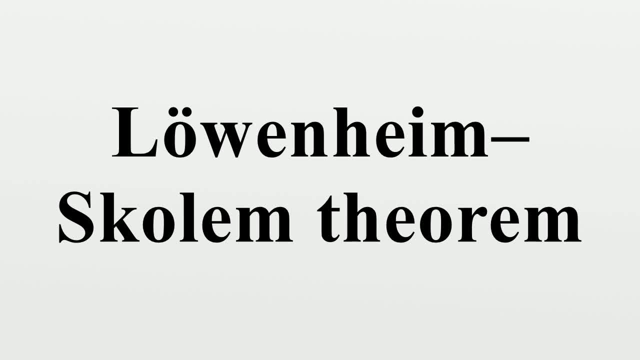 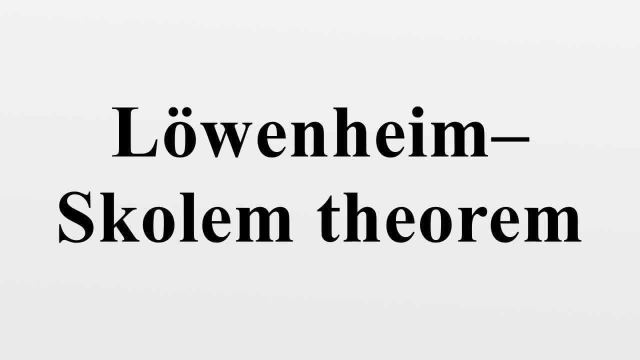 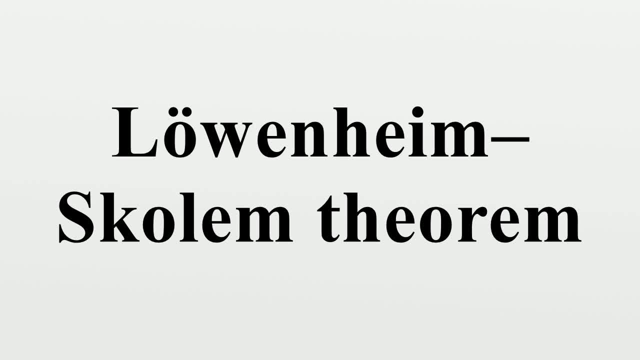 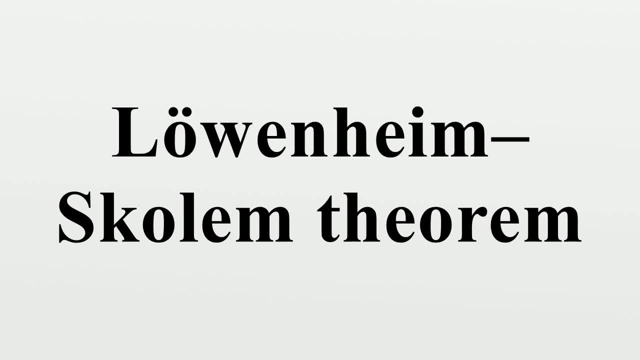 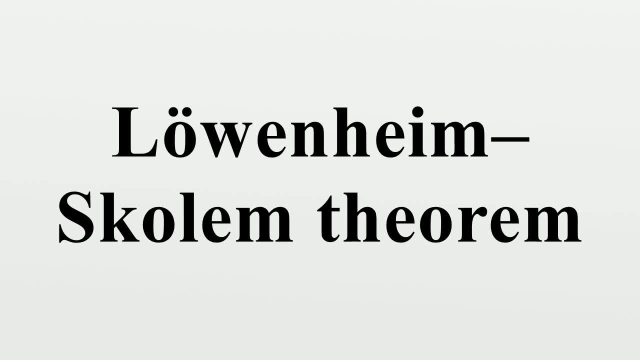 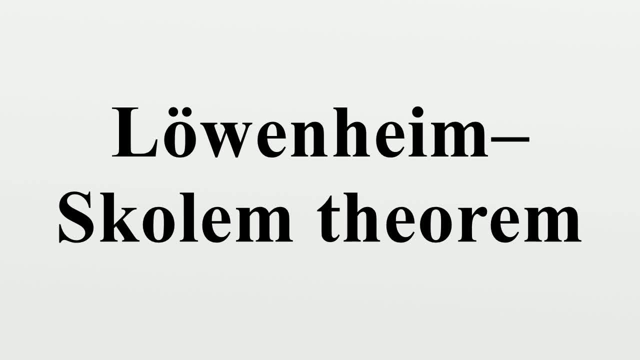 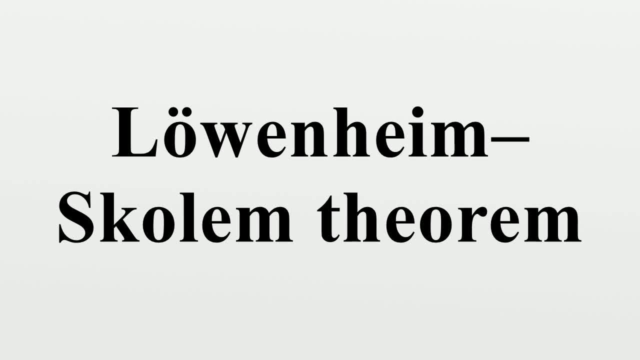 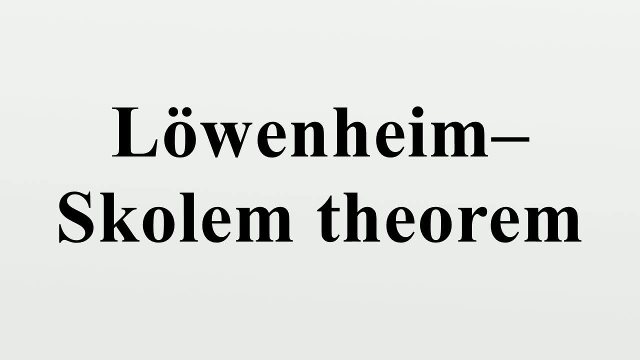 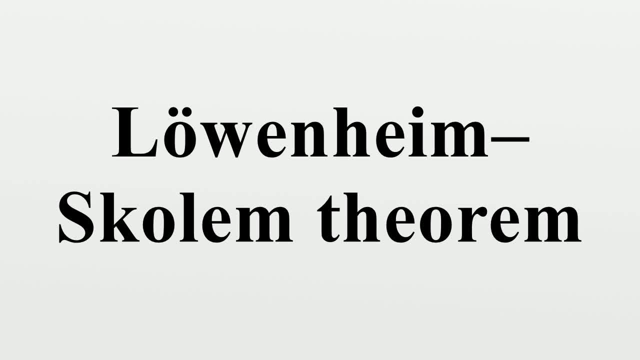 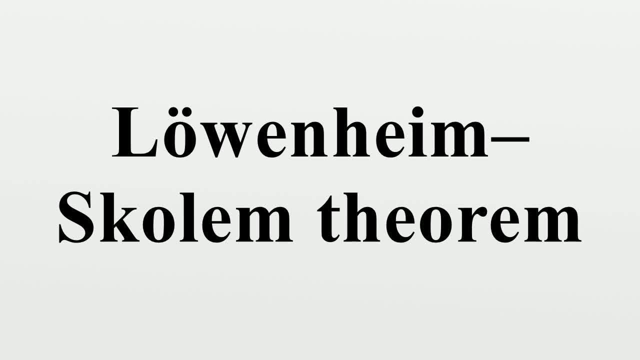 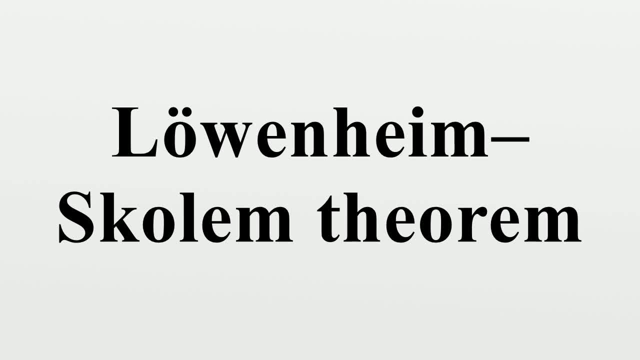 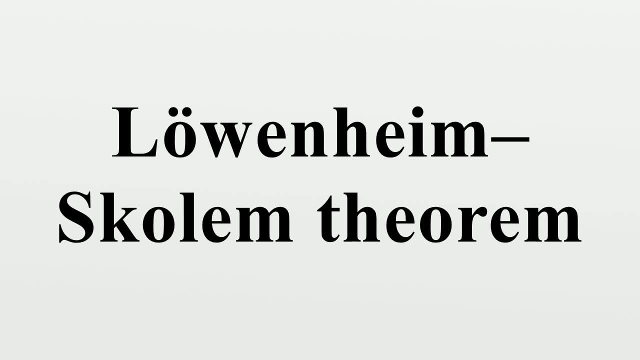 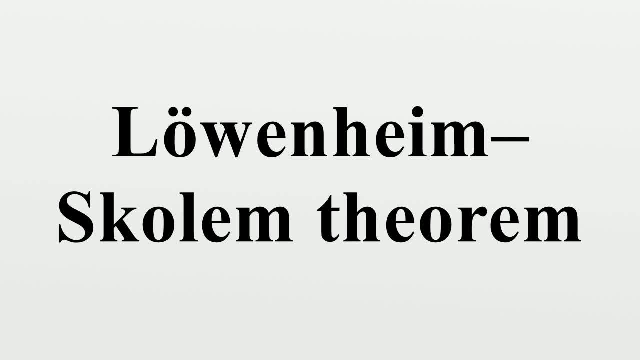 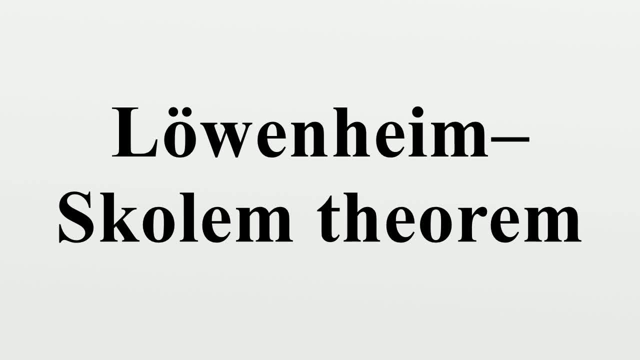 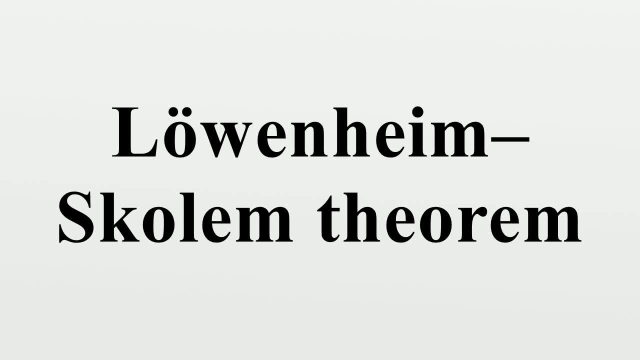 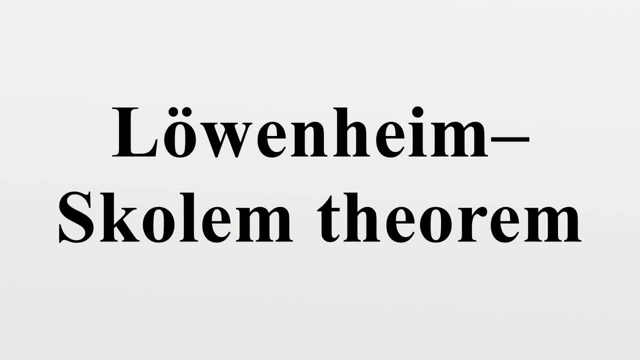 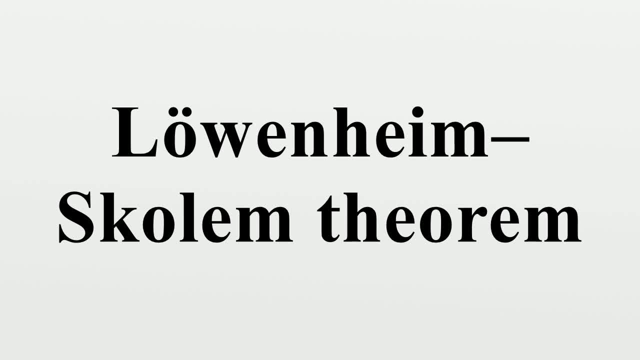